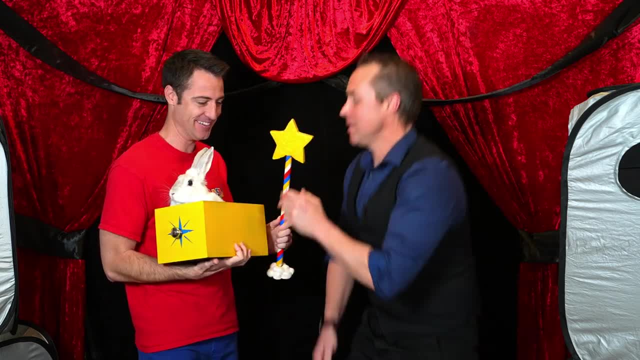 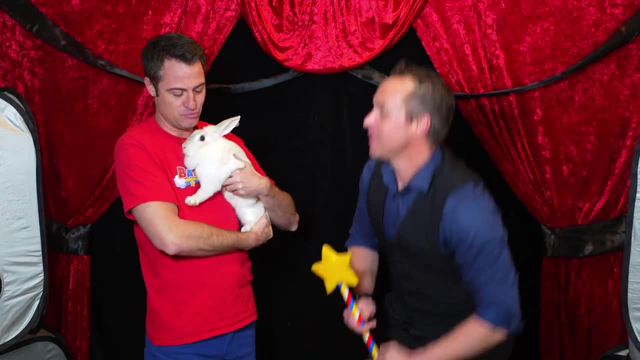 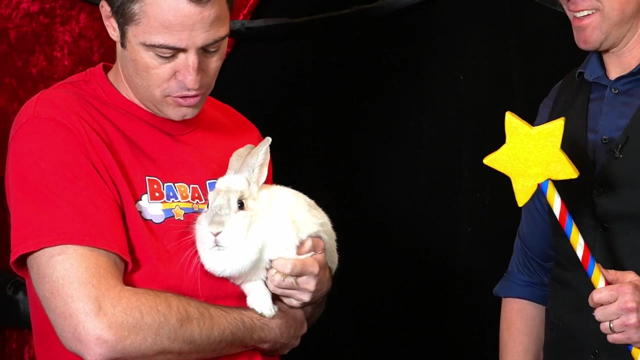 this really cute little bunny named pokus. hi, partner, can you come out of your little magic box? wow, she's really soft and cuddly. oh my gosh, can you guys see her close up? really cute. now, magic robbie, you do magic for kids all over the country. yes, how do you travel? 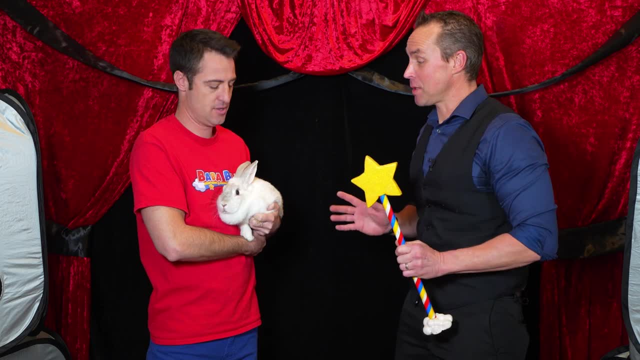 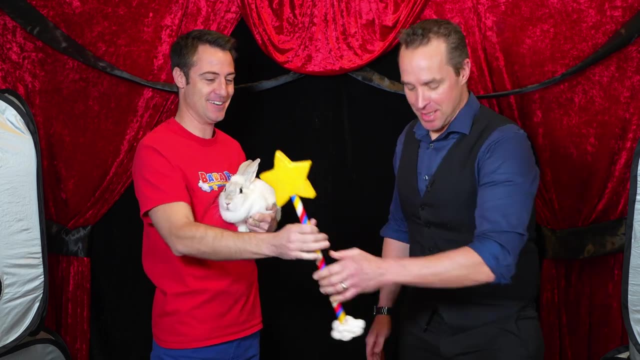 with pokus. oh, i'm glad you asked. i actually have a special magic box that makes her travel friendly. another magic box i do. all right, can you go get it? absolutely all right, i can hold the blaster, okay. what do you think pokus was thinking when she was hanging out in that box and then she appeared out? 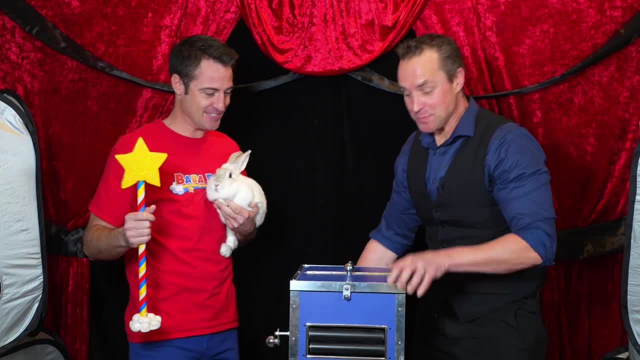 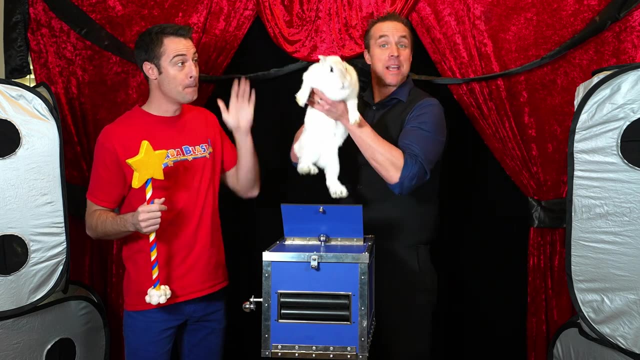 of nowhere. hi, oh, look at this magic box. this box makes any animal travel friendly, and i'm going to show you. so all we have to do is we take focus. everybody say bye to pokus, bye, pokus, all right, she goes inside the box just like this. 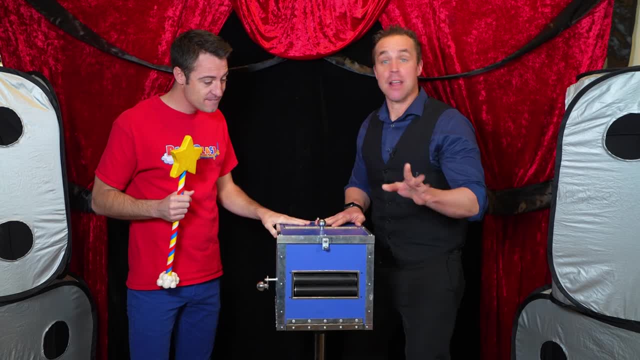 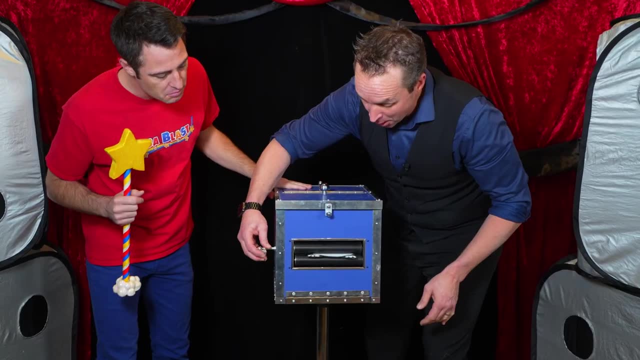 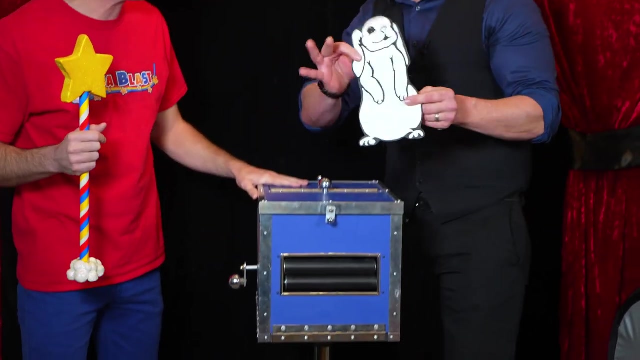 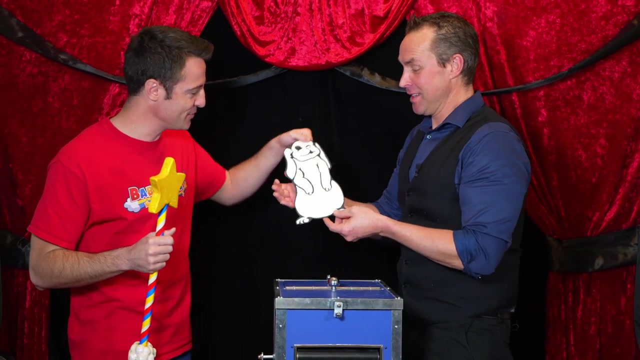 okay, now close it up. we say our magic word, which is abracadabra, just like this, and let's see what happens. oh look, focus, she is all ready to go on anywhere in the world. pretty cool, you flattened pokus into this little flat bunny rabbit. oh my gosh, now does pokus like being flat like this. 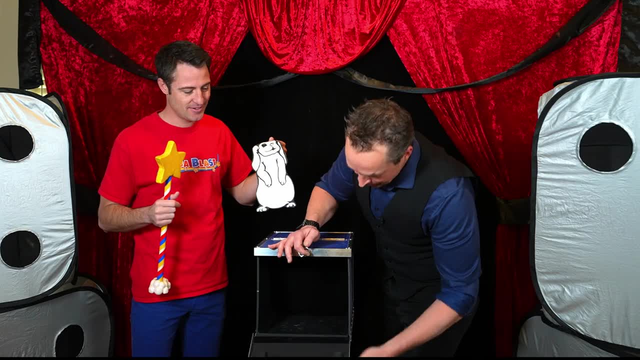 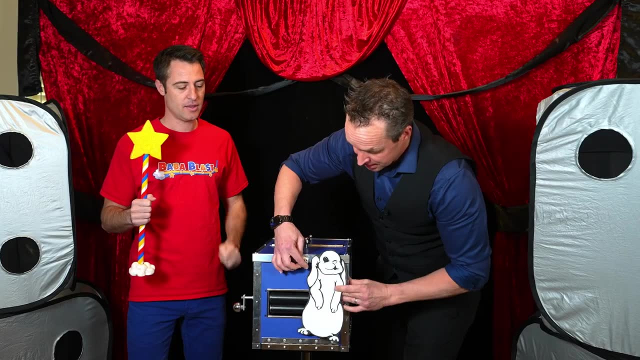 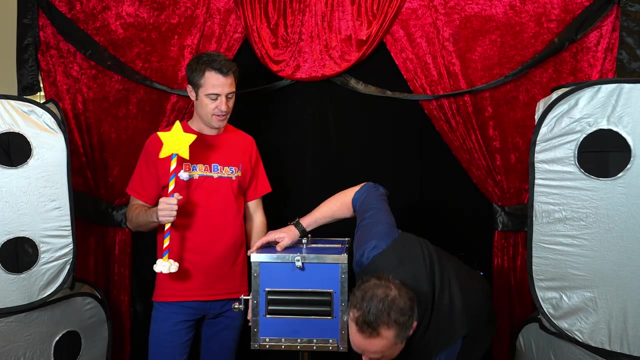 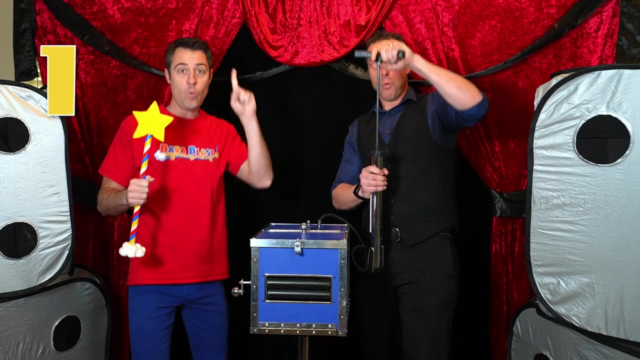 well, just for travel, let me show you. see she's gone. oh, bye pokus. so to bring her back, all you have to do is take pokus, stick her back inside the box, just like this, bye pokus, close it up and with my magic pump, let's give it three pumps. that's the magic number: one, two, three, 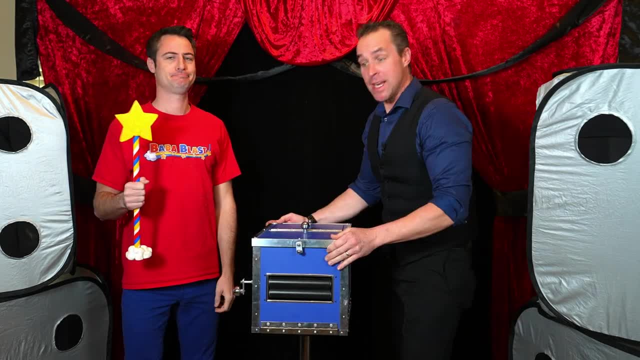 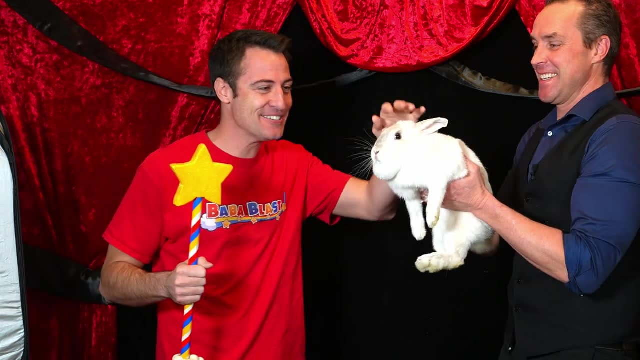 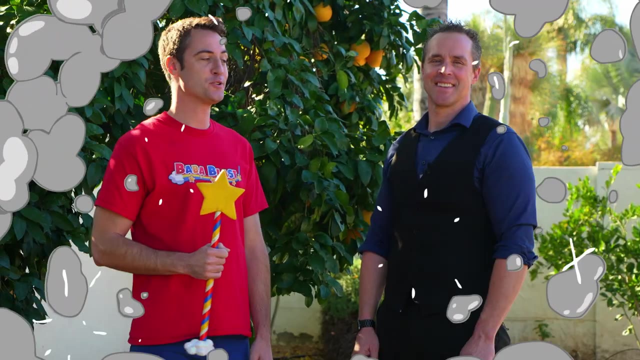 all right, and that's it. that's it, let's see ready. how cool is that? all right, that was so fun. everyone say bye to pocus and we'll be back with another magic trick. bye, bye, magic Robbie. we're ready for our next trick. very cool, I'm gonna do a trick with this piece of 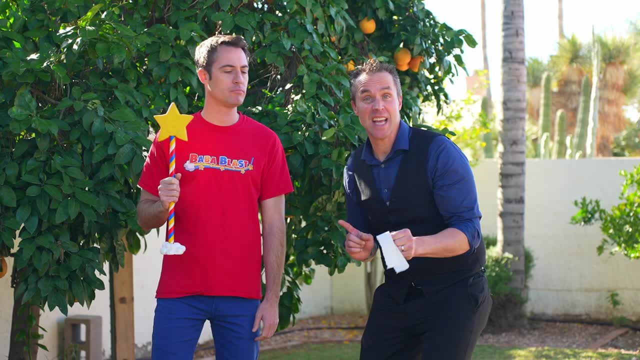 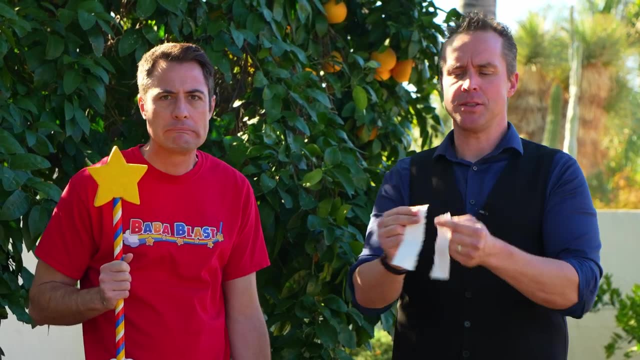 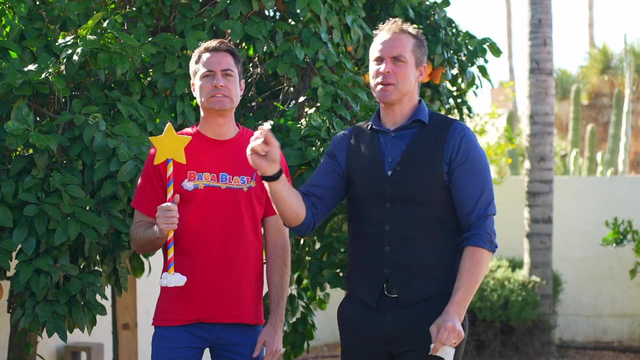 paper. now boys and girls watch the paper. this happens fast, ready, you didn't see it. okay, I'm gonna do it again a little bit slower. watch the paper. guys don't seem very impressed. I'm gonna do it one more time from a, but from up high watch. 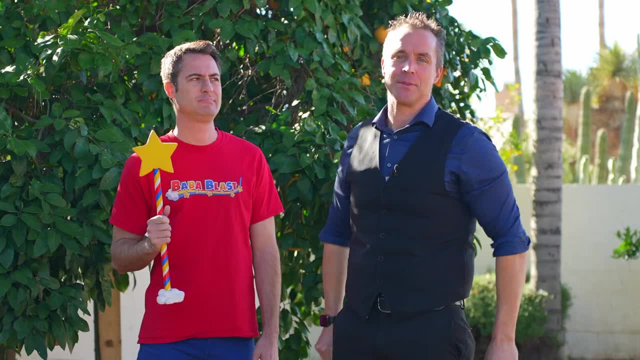 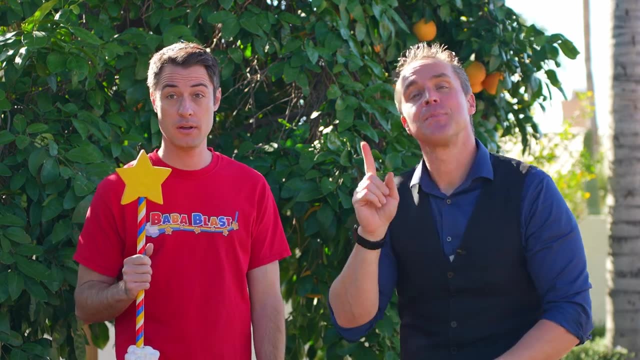 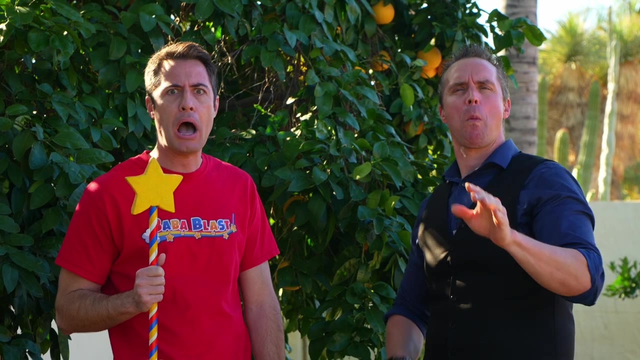 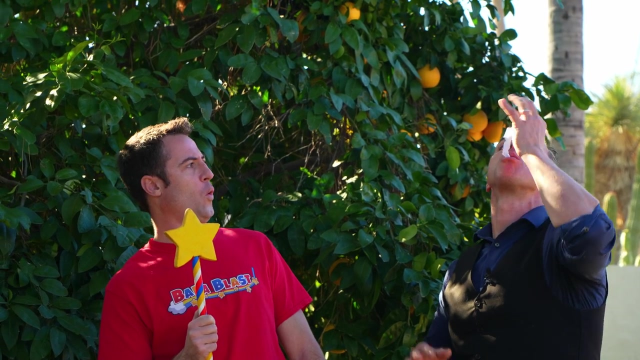 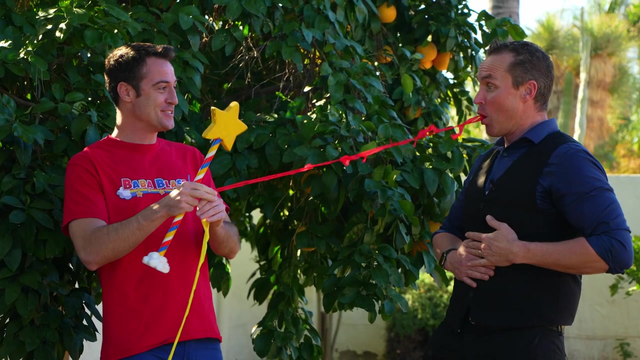 this. yeah, Wow, tough crowd, yeah, oh, this is gonna be cool. boys and girls watch the paper. now. boys and girls watch the paper. this happens, boys and girls. don't try this at home, but this should be amazing. watch this. oh, oh, oh, blaster, it's all your colors: yellow, red, yellow, red. it's still going. 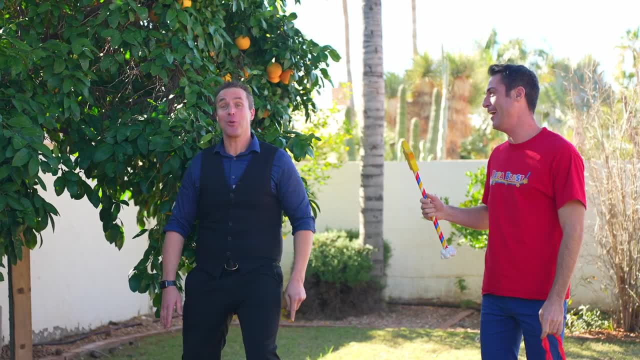 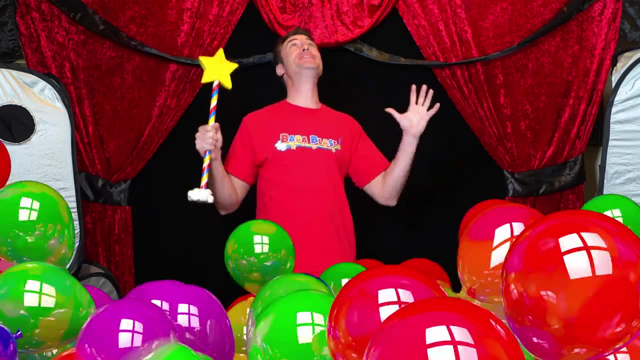 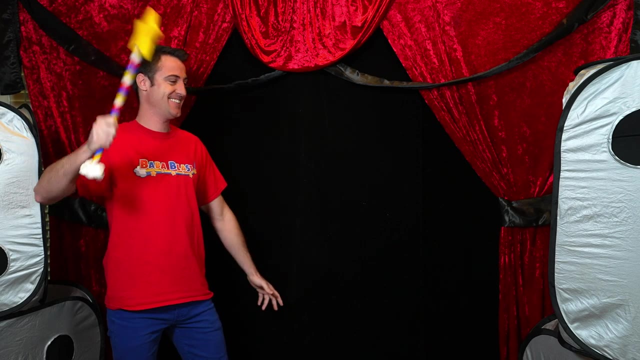 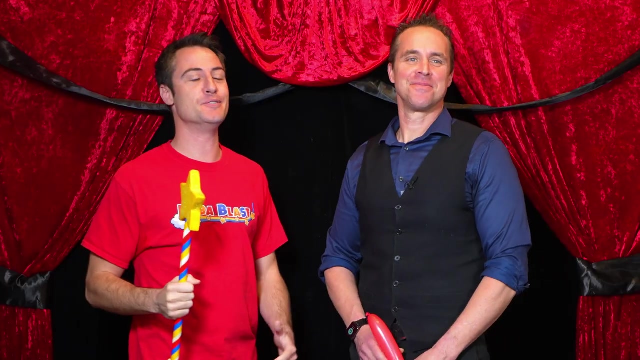 oh, oh, oh, no, oh, oh, oh, sorry, the blaster blaster. come on rounds later, alright, Jack, I love all the magic setup going on. yeah, do whatever once again, wow, wow, yeah, right was awesome the blaster and I love all the magic, but we also love, I know. 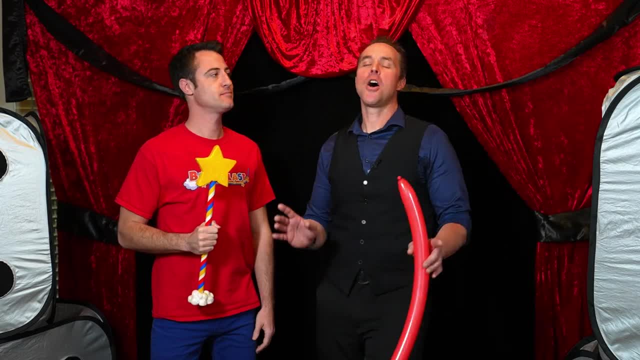 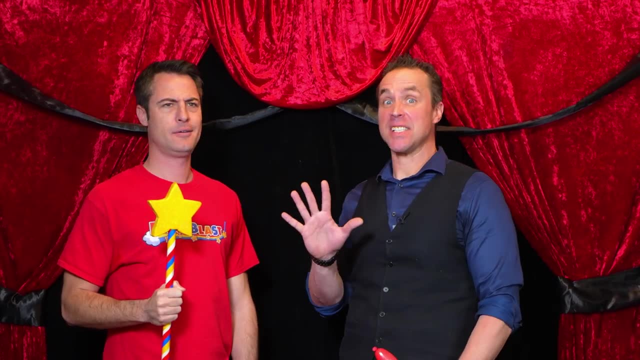 How fast can you make a balloon animal? So I have the world record right now of making a balloon dog. I can make it in five seconds. Five seconds blaster. put a clock on the screen. Let's see if he can really do this. 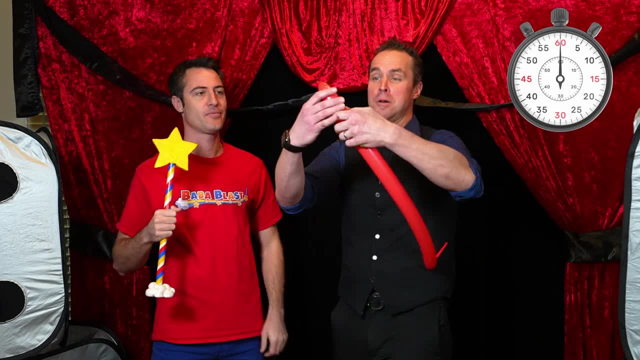 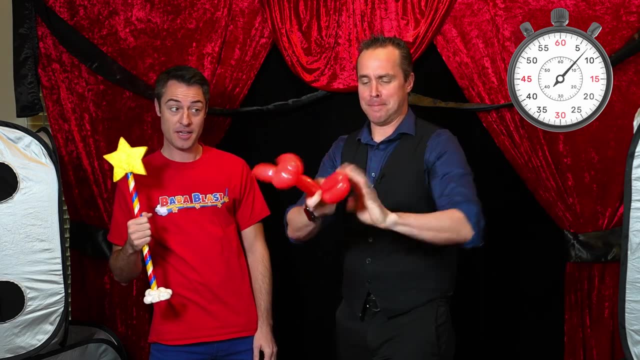 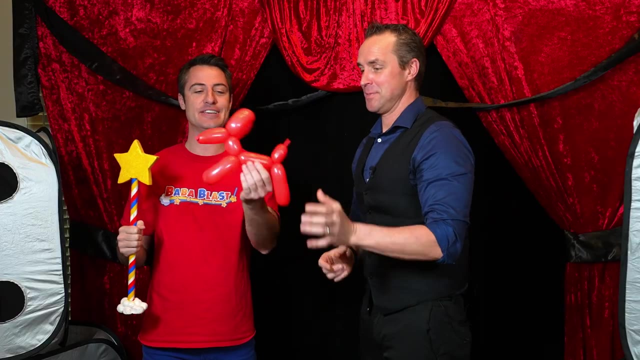 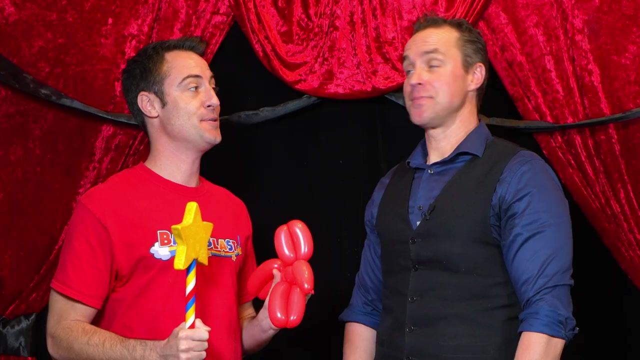 All right, are we ready? Let's go. Ta-da, nice magic, Ravi. that was great. Thank you. What should we name this little pup? That's a good name. Now can you make anything else? I can. 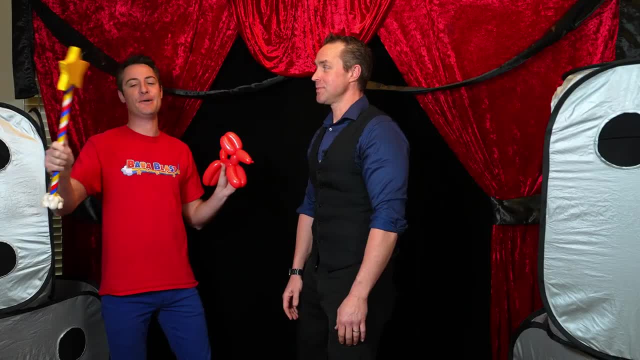 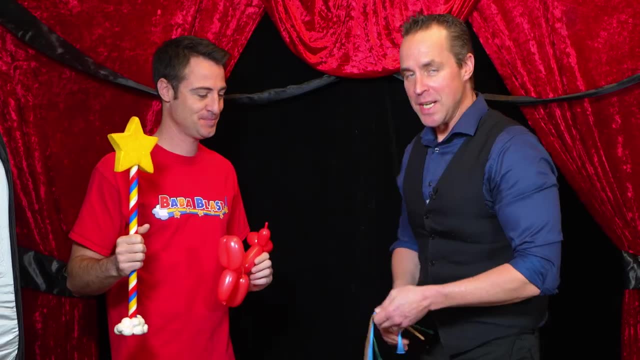 Okay, what do you need? more balloons? I do. All right, blaster, hit us up. Oh, is that enough? That is All right. great job, blaster. So we need three colors. Let's see, you guys tell me what color is this. 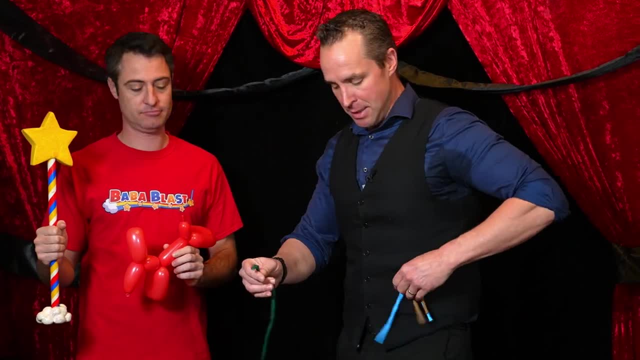 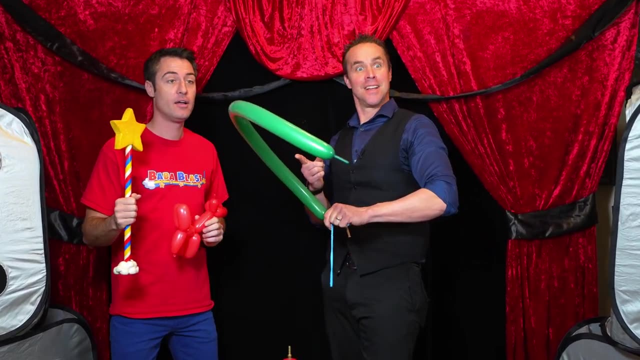 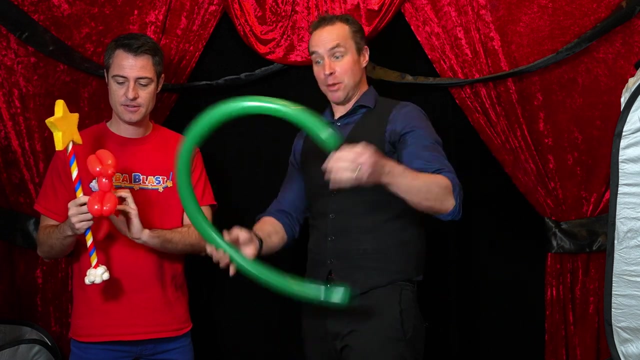 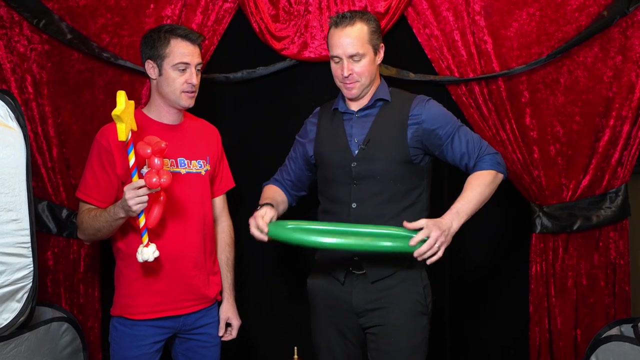 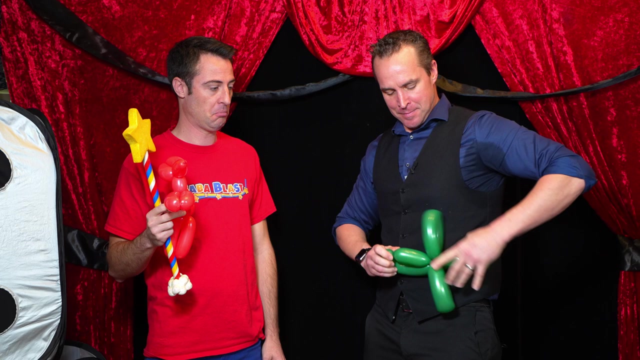 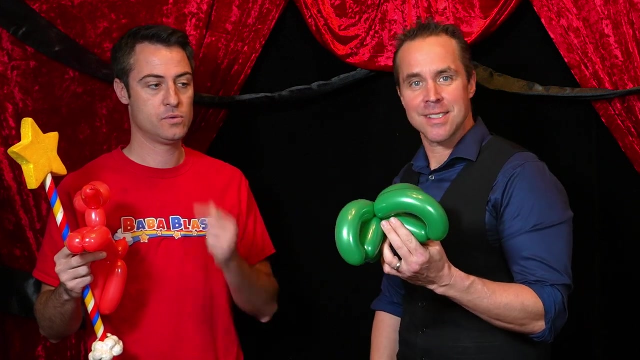 Now it might be hard to see, but you know what? Let's blow it up, then you really can see. So, Whoa, what color is that? Green, that's right. So let's do some balloon twisting. Here's the first part. can you guess what it is? 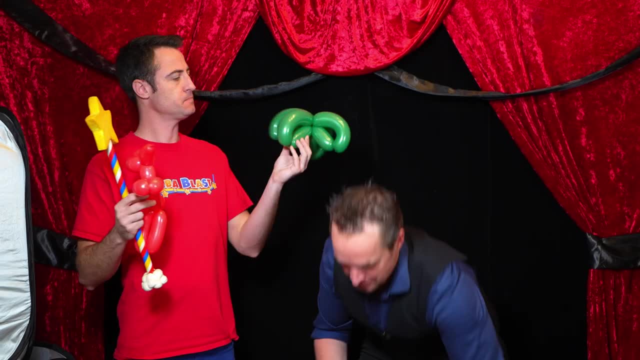 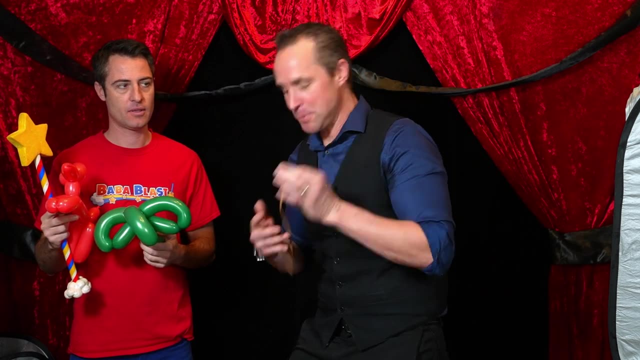 Let's do some more. Would you hold that for me, Of course, Thank you. Now, what color do you think this is? It's kind of easier to tell, but I'm going to blow it up too. Okay, All right. 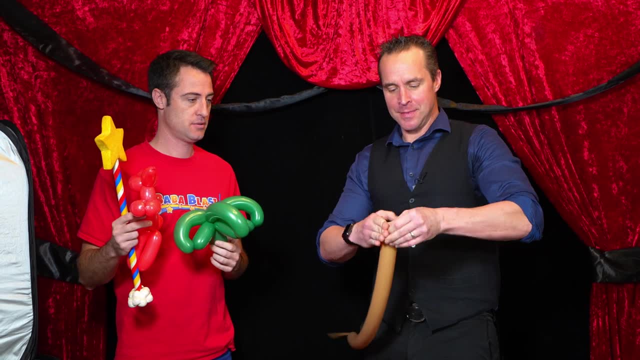 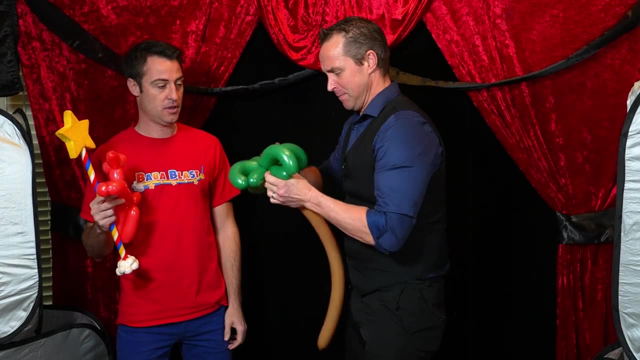 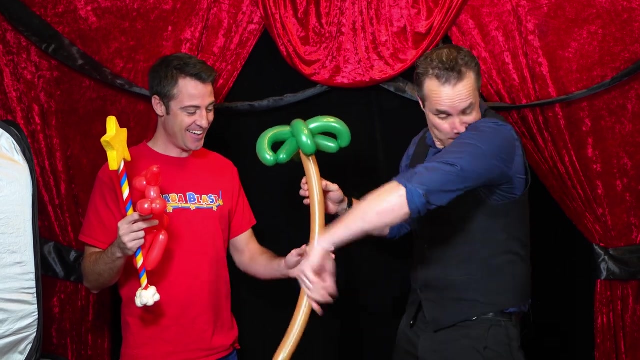 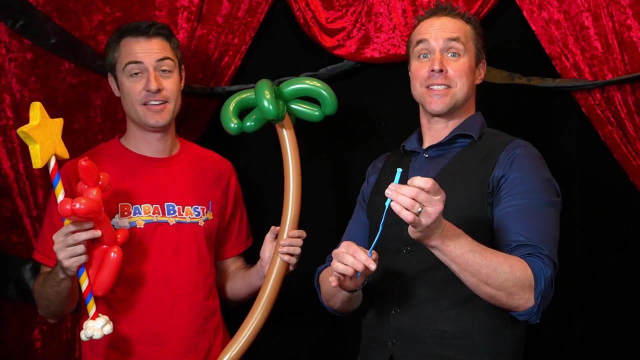 Let's see Brown Now. take this Now. can you see what it is? That's right, It's a palm tree. Nice, This is great. There's more to it. There is one more thing. Can you guess what color this is? 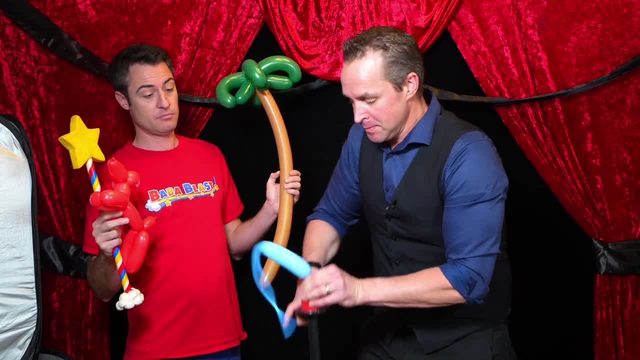 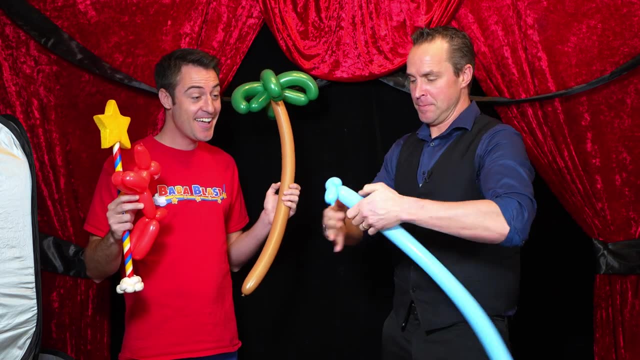 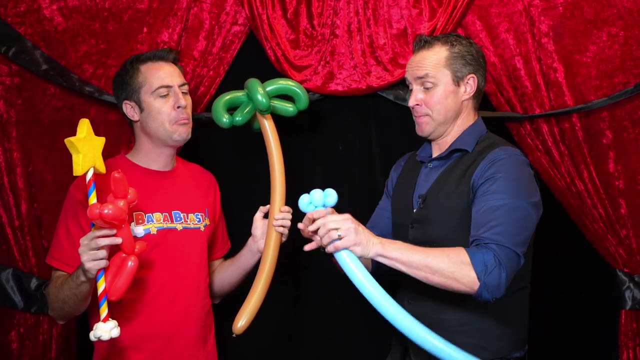 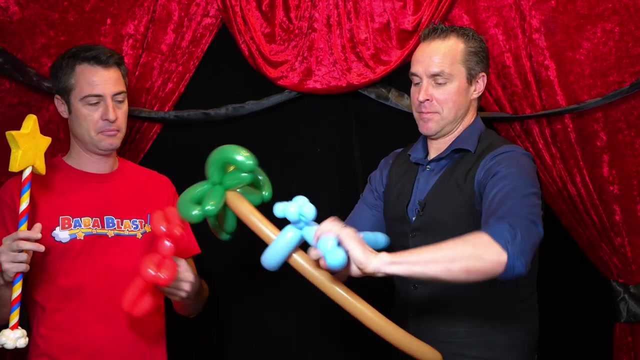 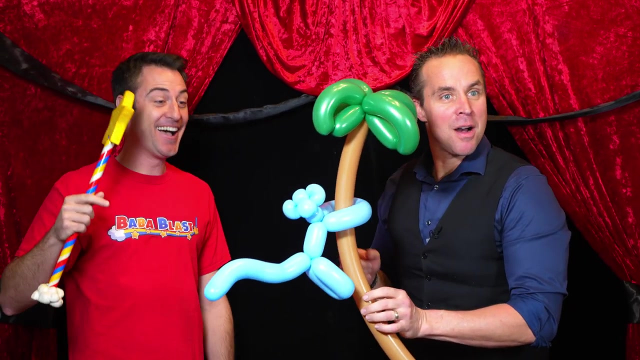 That's right, It's blue Whoa, That's right, It's blue Whoa. Cool Ready, There's the head. Look what it is. It's a monkey in a palm tree. You know what? It's kind of missing something. 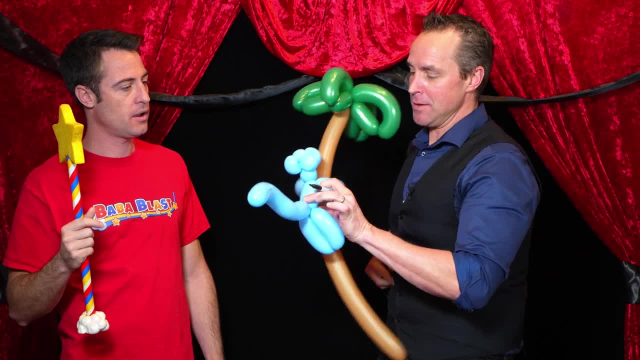 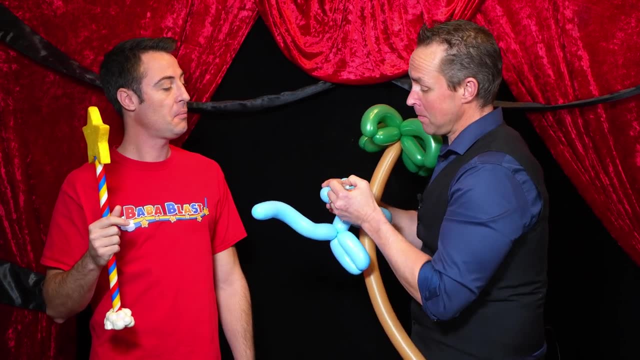 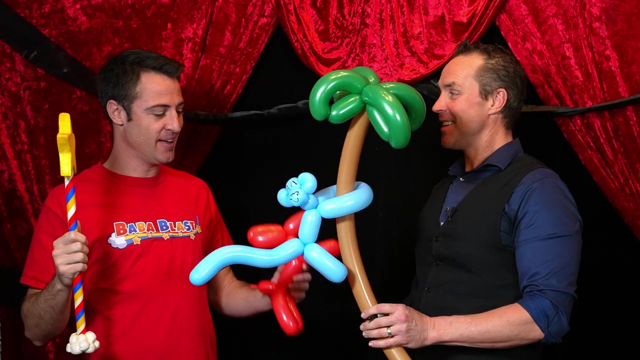 Oh, it needs a face. Let's draw a face on there. It's a happy monkey on a palm tree. Great job, Magic, Robbie. Hey, well, with our monkey and our dog, we can have a lot of fun, Blaster. 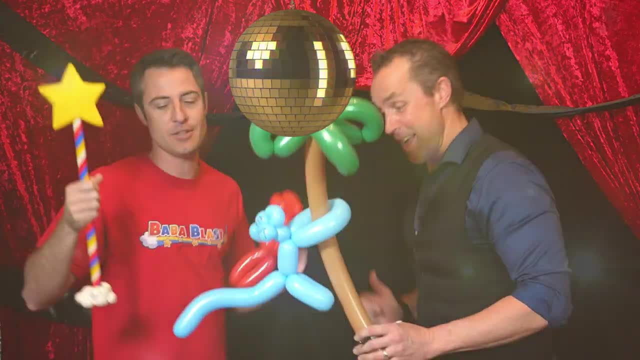 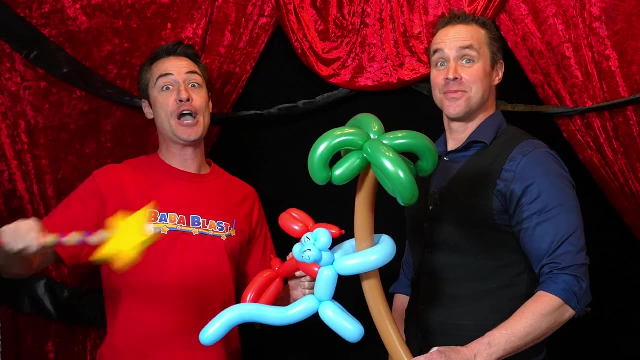 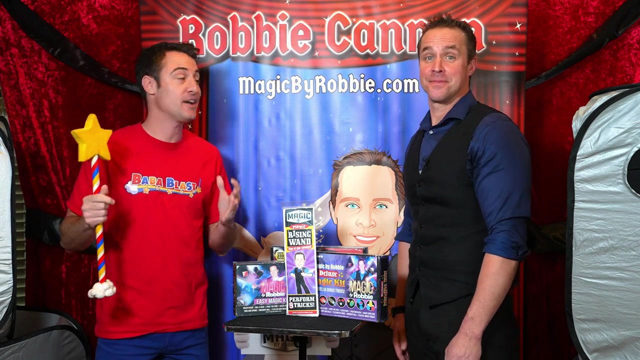 How about a quick dance party? Hey, but there's even more magic to be had. So let's go The Blaster, and I think it's so cool that anybody, young or old, can become a magician. How old were you when you became a magician? 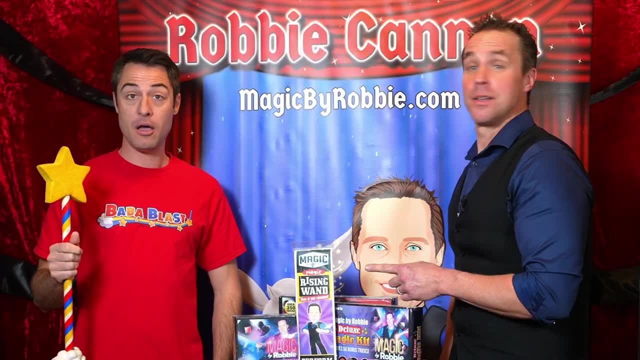 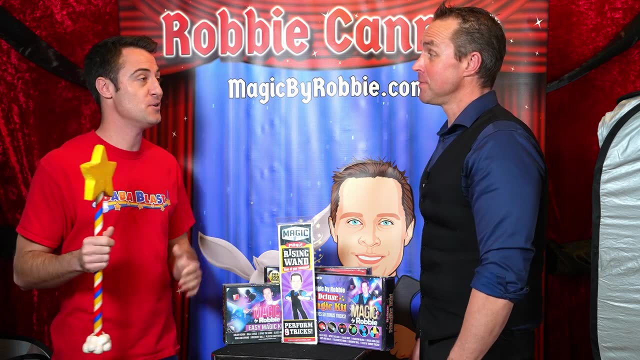 So I became a magician when I was eight years old. Wow, I did. And I did my first magic show when I was 13.. Wow, So you've been a magician for a long time and you started really young I did. 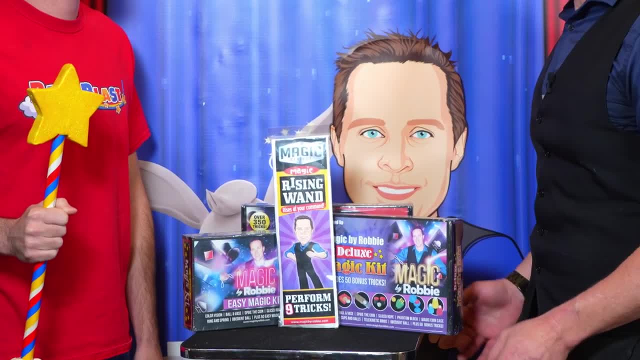 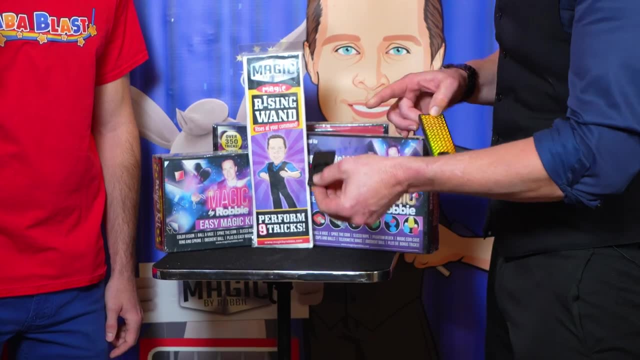 What were some of the first magic tricks you learned? You know I have some right here. Great, Let me show you. Look what I have here. It's this little box, You see it. It's got a hole inside there big enough for a quarter. 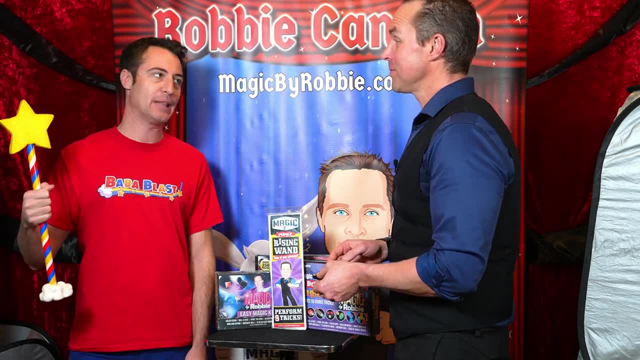 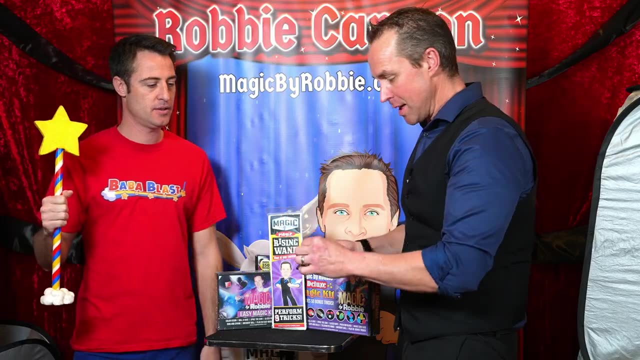 Do you happen to have a coin on you? I don't, but Blaster. Hey, perfect Blaster, Here's a quarter. Thank you. Now we're going to take the quarter and stick it inside the box, just like that. 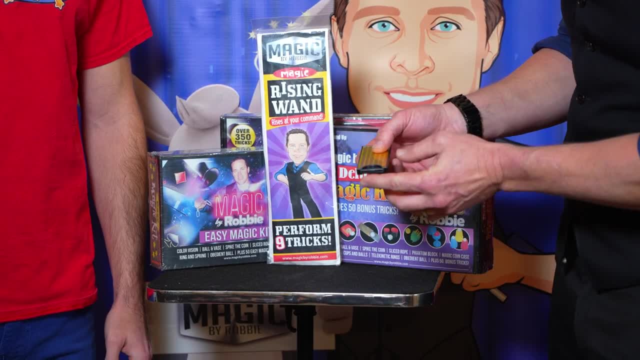 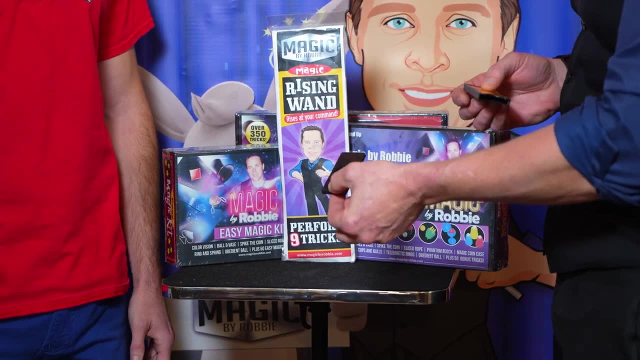 Now Put it inside the box And one, two, three. Oh, it disappeared. It did. I don't like it when my money disappears, though Magic Robbie Me either, So let's see if we can bring it back. 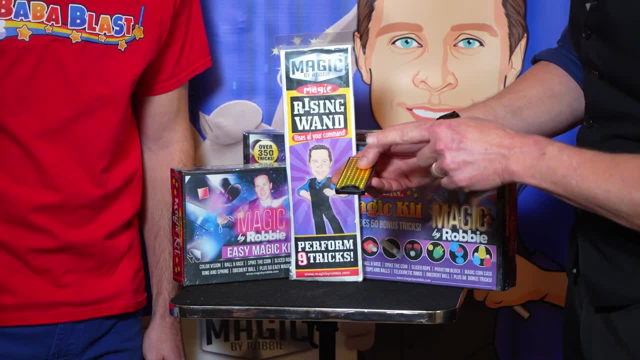 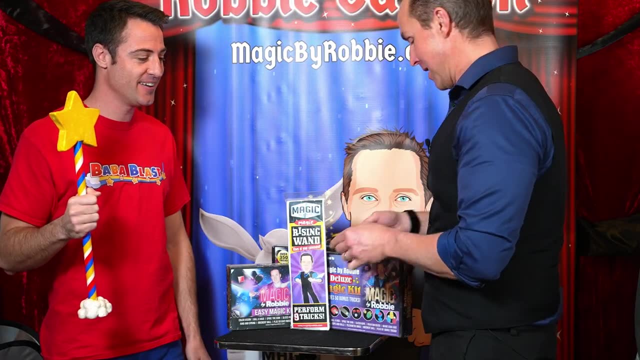 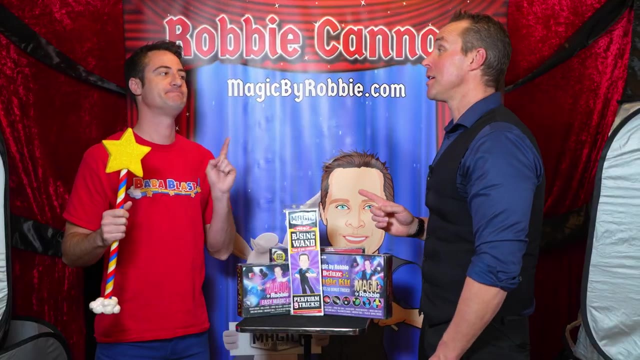 OK, Wow, Wow, It came back. What a great trick. It is very cool And Magic. Robbie, how did you do that magic trick? Now, I can't tell you the secret, but you can learn secrets too by getting one of my magic kits. 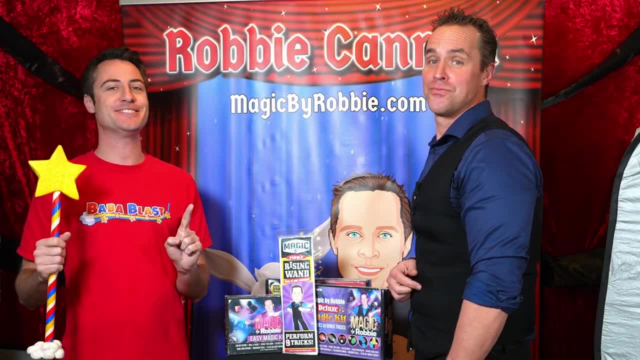 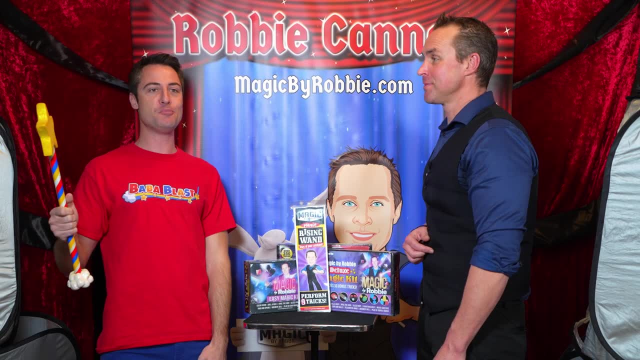 That's right, because a magician never tells their secrets. Now, I love these magic kits, Magic Robbie, but I want to see some more magic. Can you help us out? Absolutely, All right, let's go do more magic. A box. 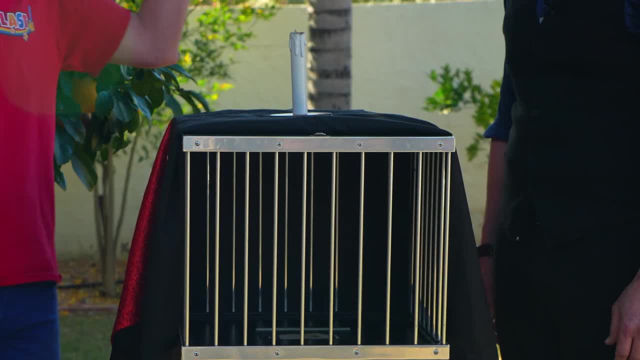 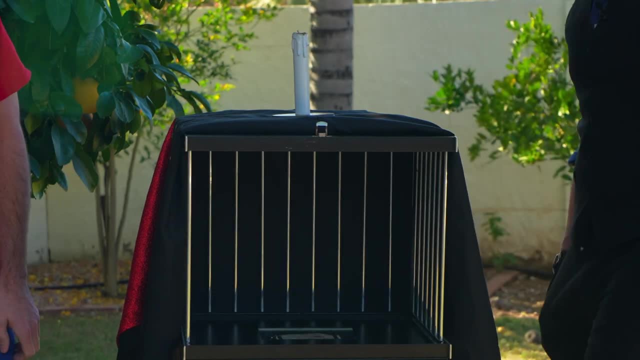 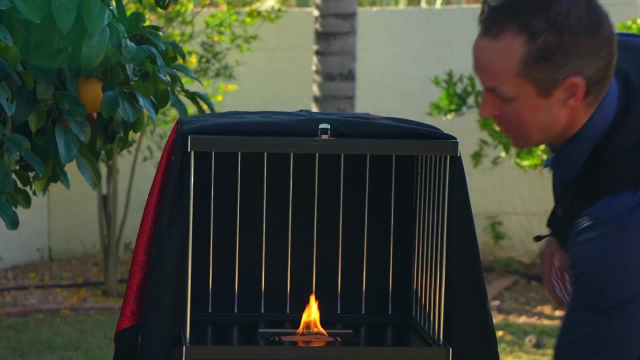 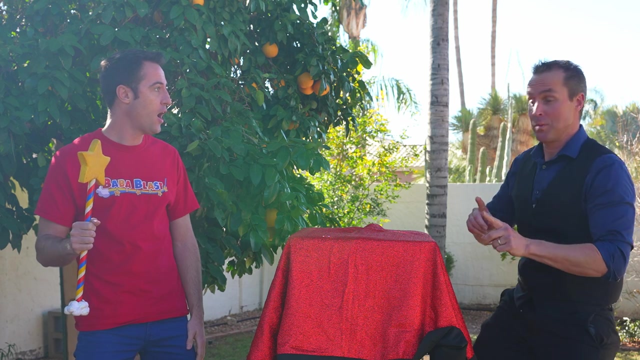 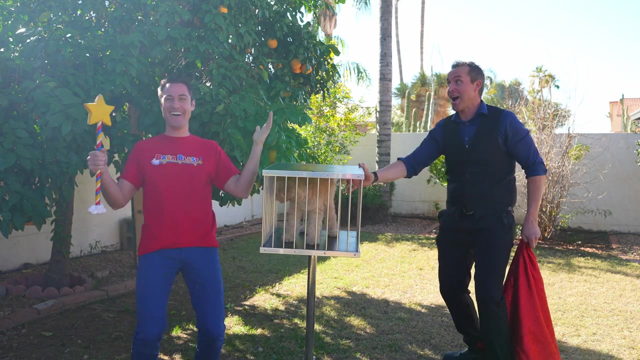 Bars. A candle Magic. Robbie, I'm lost. What are we doing? I would love to show you. Check this out. Watch the candle. Whoa, Oh, Hi there, How cute. This is my magic. This is my magic. 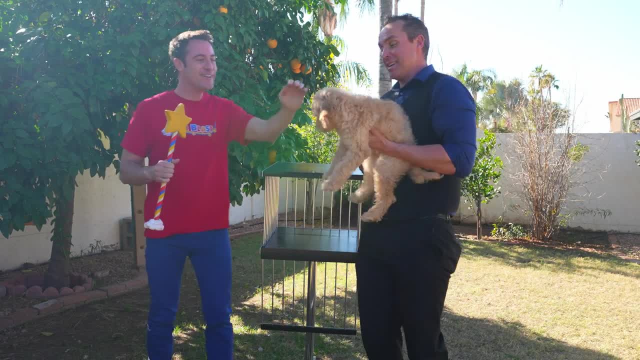 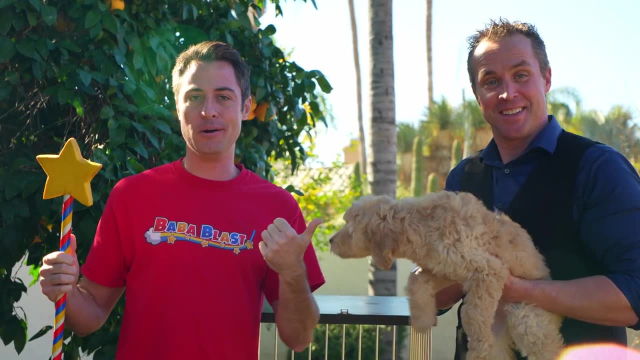 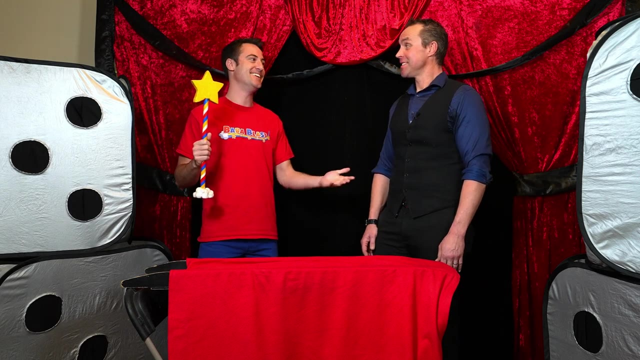 This is Lily. Out of the fire comes Lily. Oh, you are so precious Man. magic is awesome. Sometimes you get to meet a really cute puppy dog. Let's go see what else we got: Magic Robbie, Magic Robbie. what's going on here? 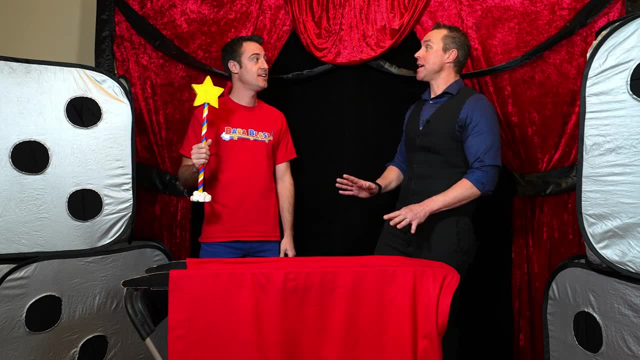 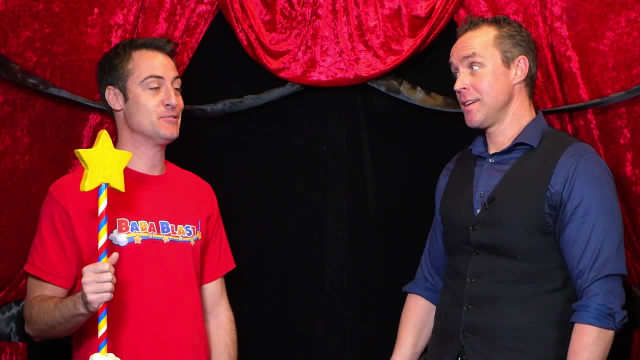 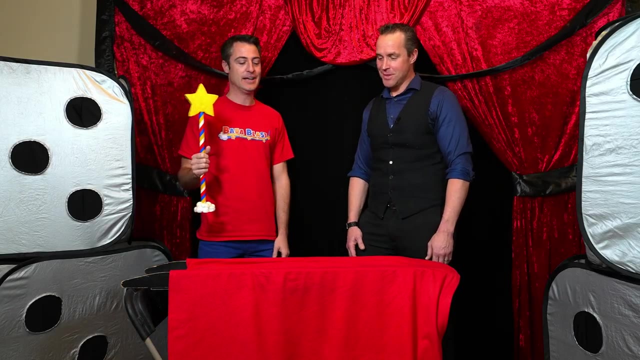 I'm glad you asked. You know, I think we should make somebody float. Float, Yes, Would you like to do it? That sounds like a job for somebody who's not afraid and really brave. And besides, Magic Robbie, I'm too big to lay on this and float. 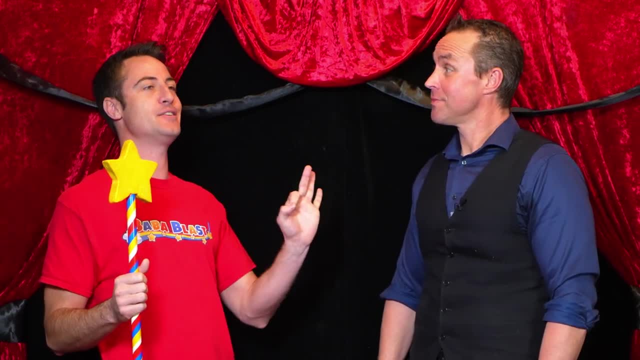 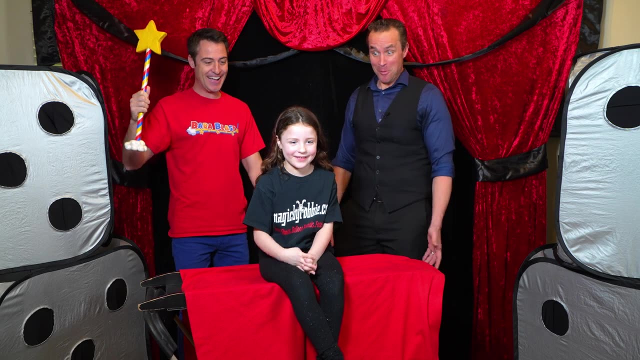 You're right, But you know what? I think the Blaster can find the perfect magician's assistant. Blaster, can you help us out? Whoa, Hi there. What's your name? McKenna, It's the magical McKenna. 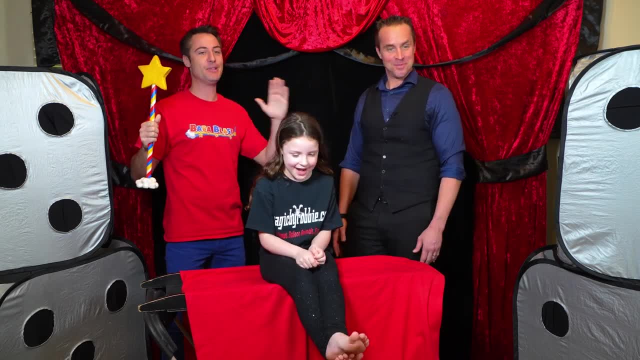 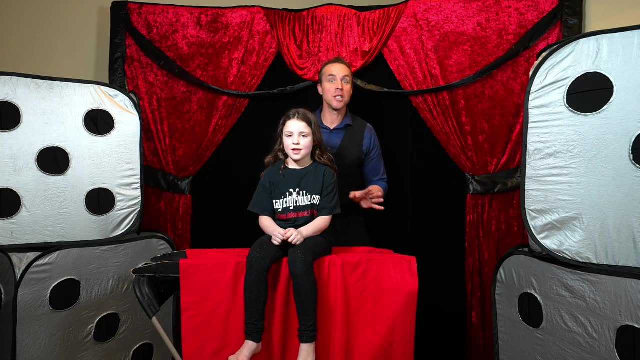 Robbie, you have your perfect magician's assistant. I think the Blaster and I are going to go watch with our friends. OK, All right, Here we go, Let's go. Now we're going to do a little bit of magic with McKenna. 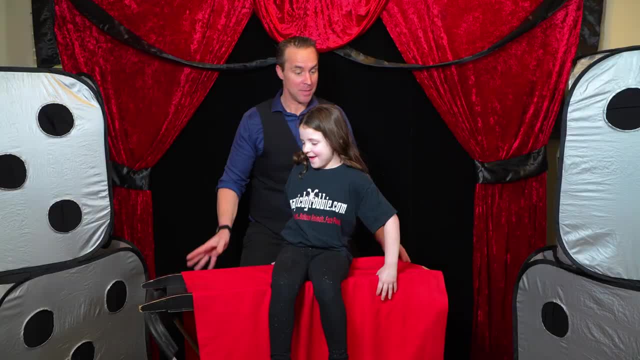 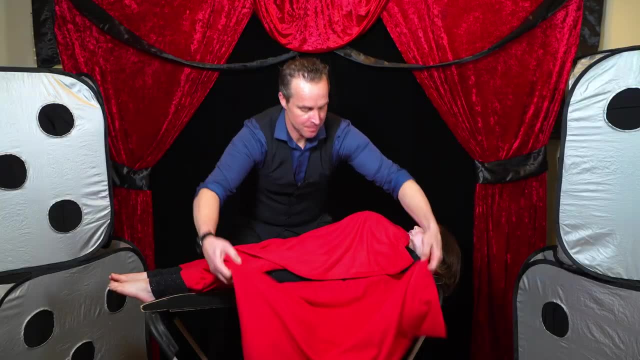 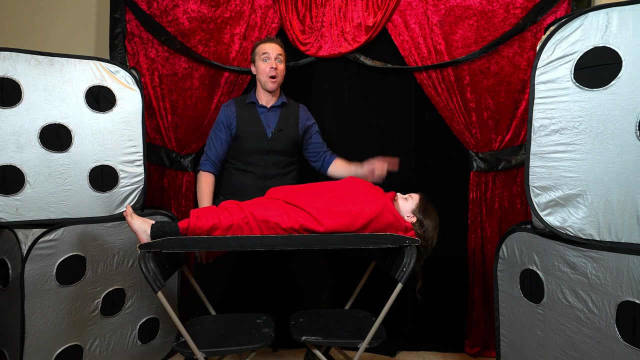 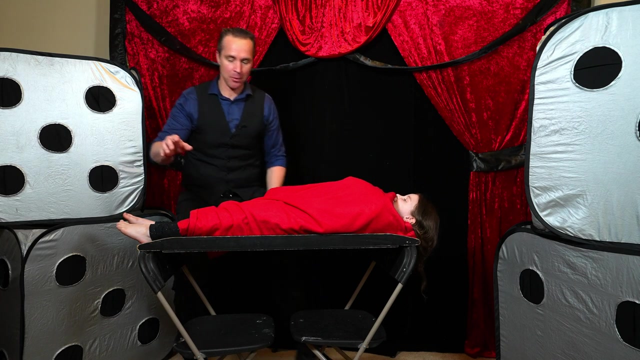 Are you guys ready? Here we go, McKenna, lay down for me please. All right, boys and girls, let's count to three and do some magic. Here we go. One, two, three. Nobody move. Check this out. 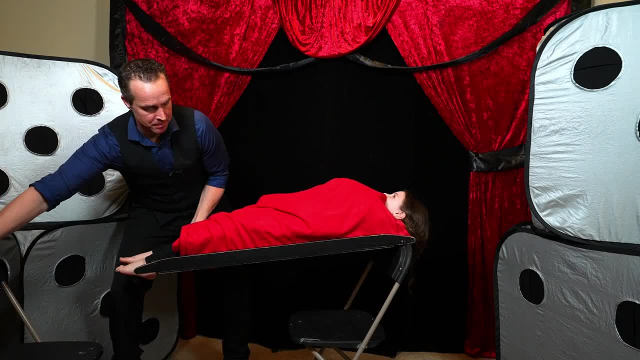 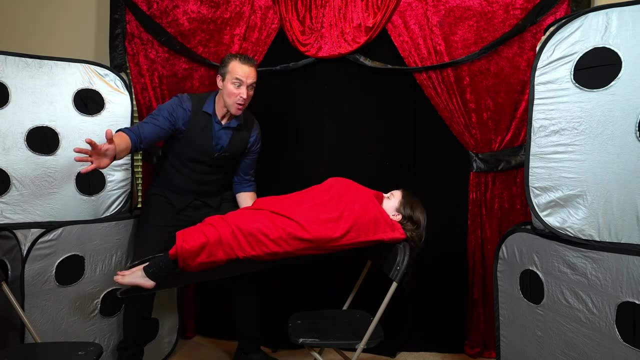 See if they know that we have a magic wand: One, two, three, One, two, three, And now we are going to spin a ball. Wow, She's floating Cool. Hey, McKenna, How do you feel?